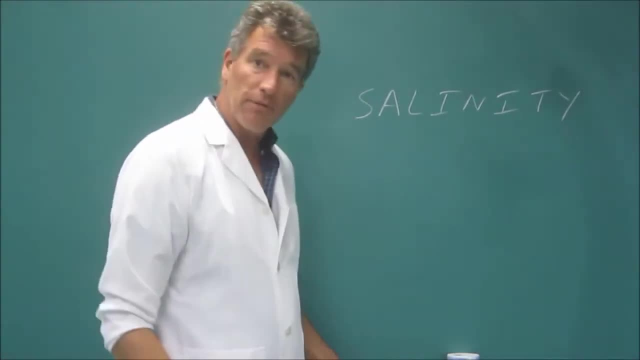 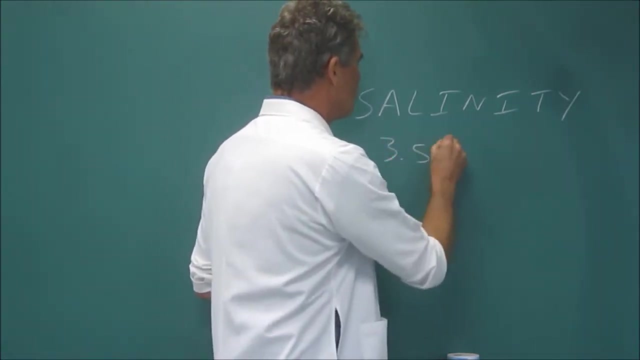 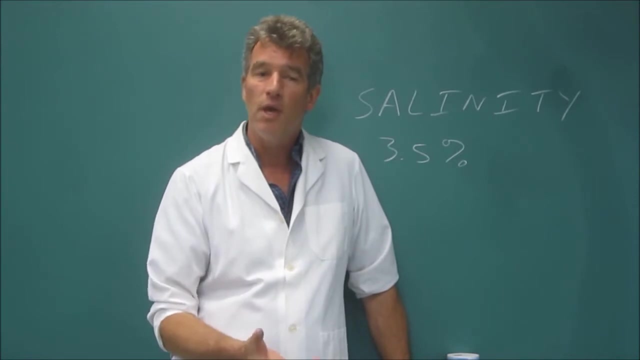 In any event, we measure salinity using a couple of different measurements, And the average salinity of ocean water is 3.5.. What that would mean is if you could imagine a tub of water that weighed 100 pounds, if you let the water evaporate, you'd be left with about 3.5 pounds of salt in the tub. 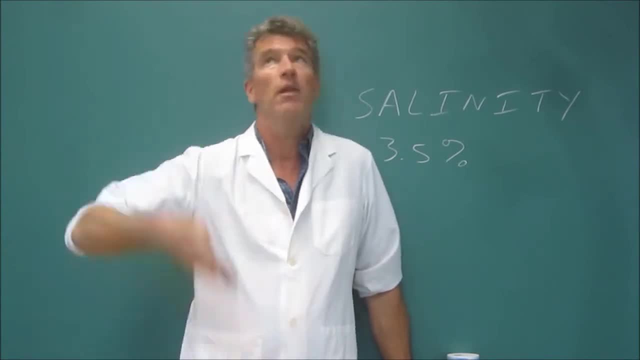 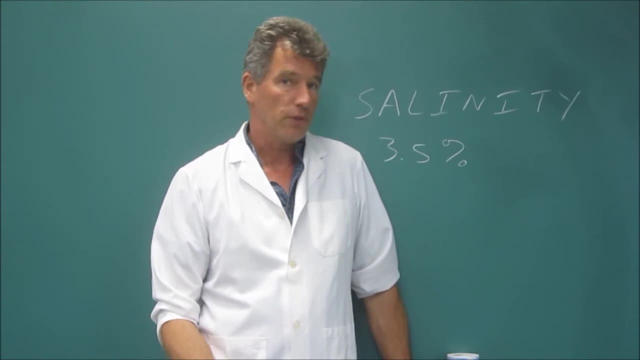 Which means that 96.5 pounds of water molecules evaporated and went into the air. Now in oceanography we actually use a different measurement for salinity. more commonly than percent, We use what's called parts per thousand. If you think about it, a percent is just out of a hundred. 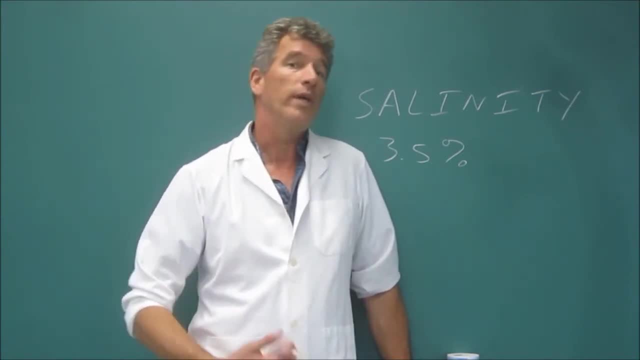 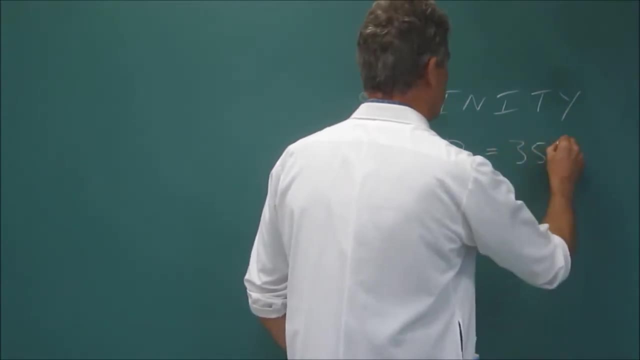 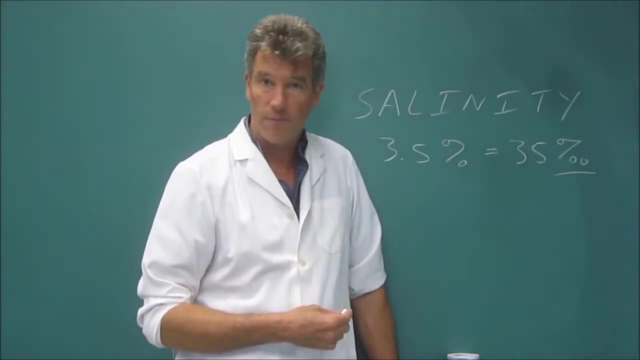 If you say 10%, it's 10 out of a hundred. Well, we can also say how much out of a thousand, And it turns out that 33.5% is the same thing as 35 parts per thousand, And we write it that way, like a percent sign with a little extra zero underneath. 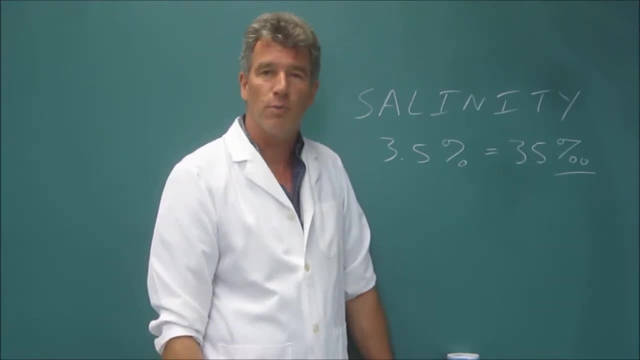 And so these are equal to each other: 3.5% or 35 parts per thousand, They're the same. In your lab, you're going to be making your measurements and writing down your data in parts per thousand, And the samples that you might be dealing with might have only one or two parts per thousand salt. 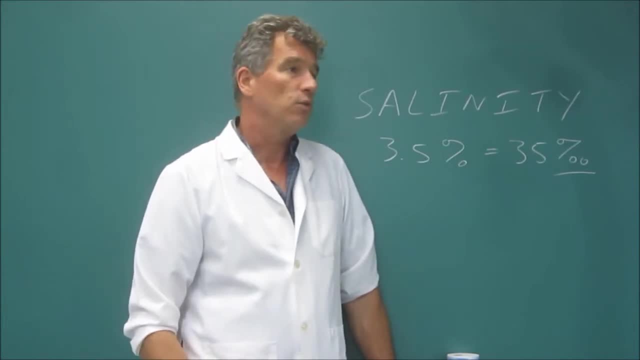 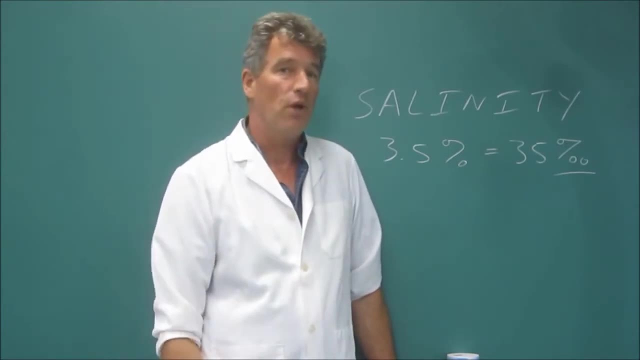 or they might be up to close to 40 parts per thousand. That's the range of salinities that we can get, going all the way from, say, a river which is almost entirely freshwater to some of the saltiest parts of the ocean. 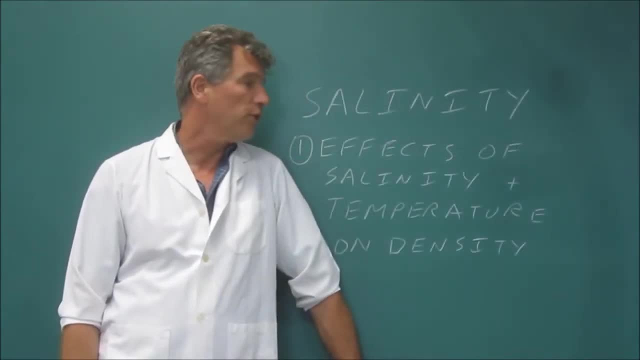 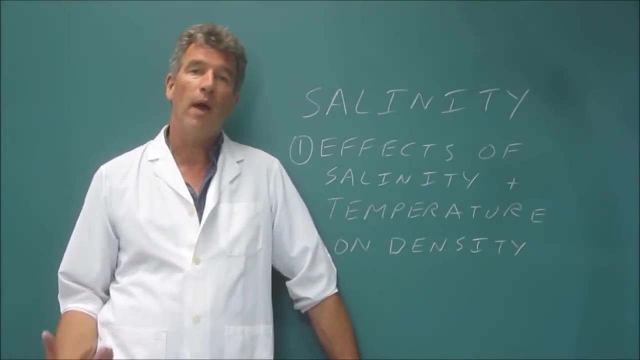 The first thing you're going to do in the lab is explore the relationship between salinity and temperature and water density. The density of ocean water is affected both by its salinity- how much salt is in the water- and also its temperature, And this is important because the density of water controls how the water moves. 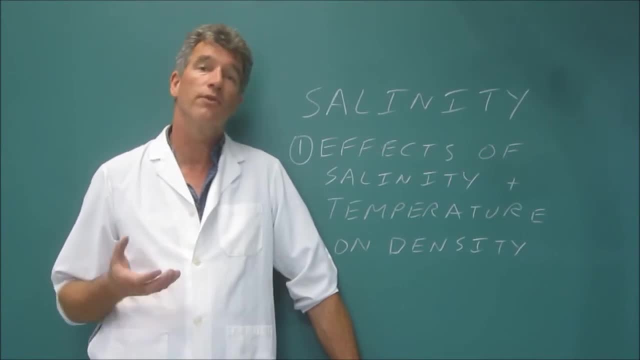 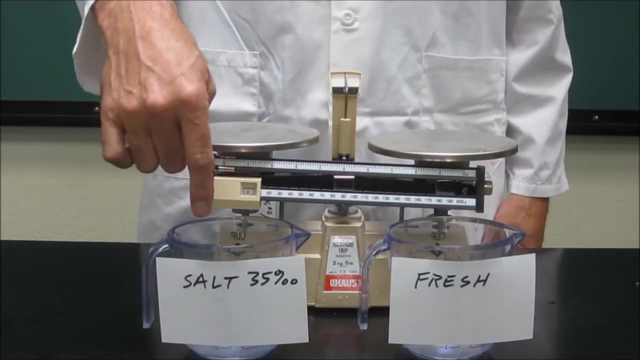 In general, less dense water will tend to float up near the ocean surface and more dense water will tend to sink. I'm going to show you a demonstration now, exploring the relationship between temperature, salinity and density. I've got two water samples here: fresh water and then some ocean water: 35 parts per thousand. 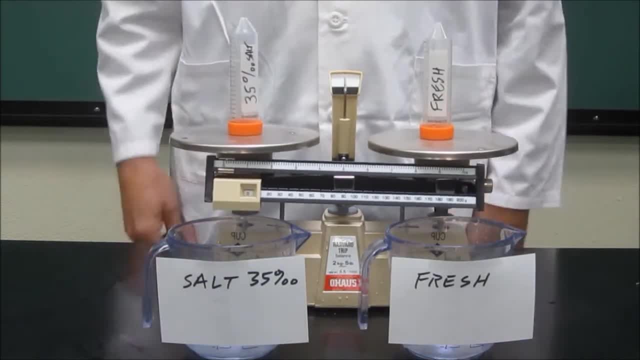 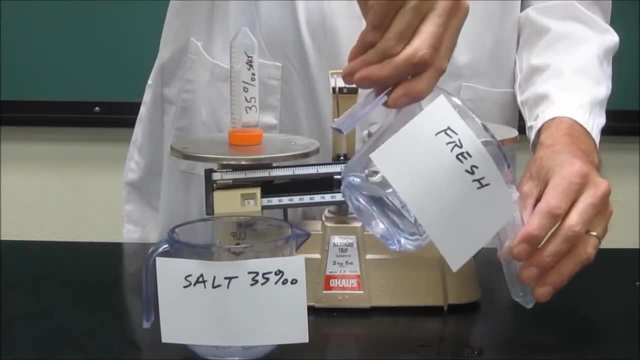 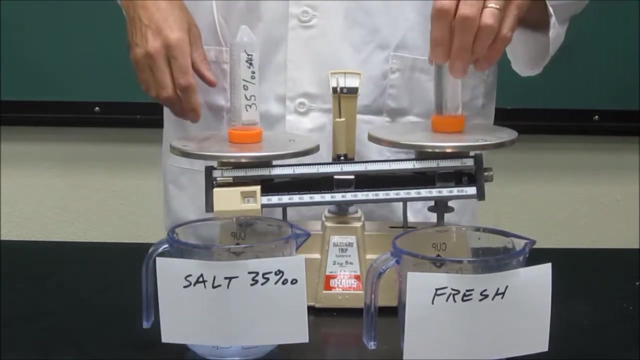 And I've got two containers here And you can see these two containers weigh the same And I'm going to fill this container with fresh water right to the brim, so there's no air bubbles there, And I'll put it on the scale and fill this one with the salt water or ocean sample. 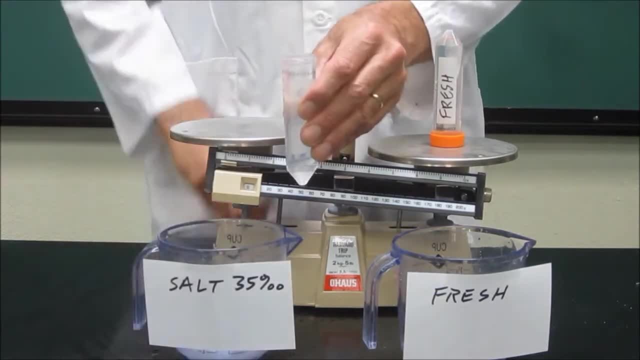 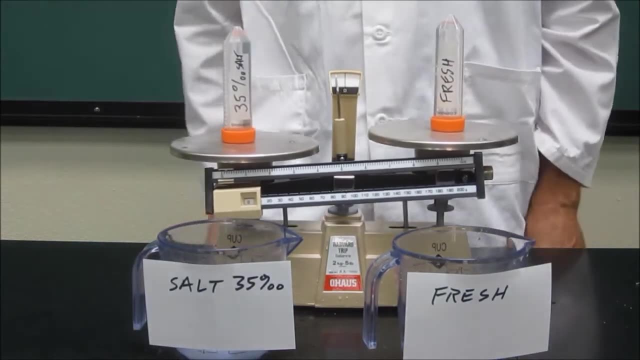 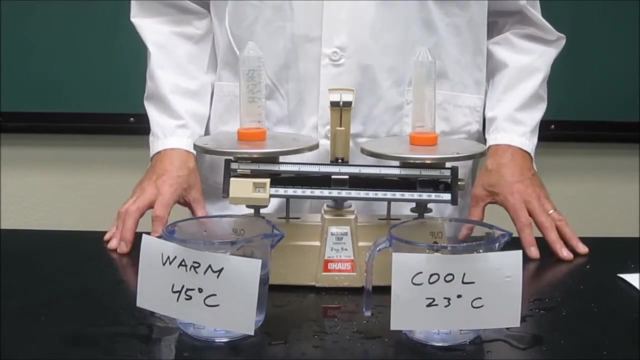 And put it on the scale And you can see that's the salt water. And you can see that the salt water is heavier, It's denser, which means heavier for a given amount. Now we're going to look at the effect of water temperature on the density of water. 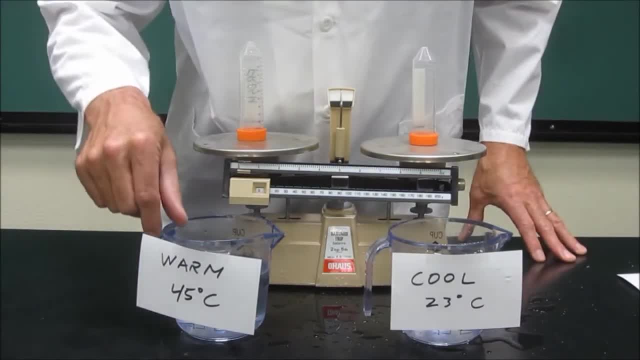 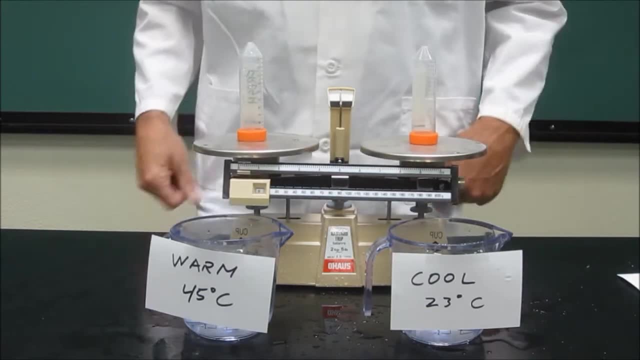 I've got two water samples here: a warm water sample 45 degrees Celsius and a cool water sample 23 degrees Celsius. That's actually just room temperature And you can see the two containers here on the scale are the same weight. 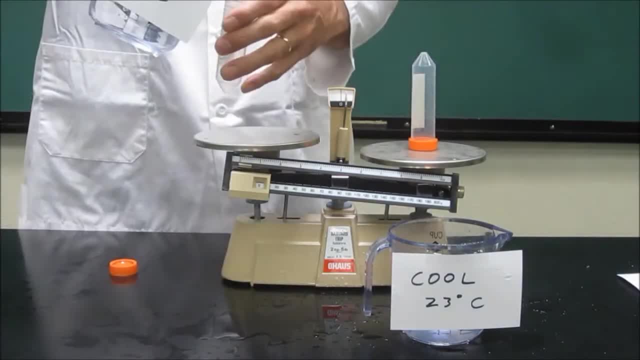 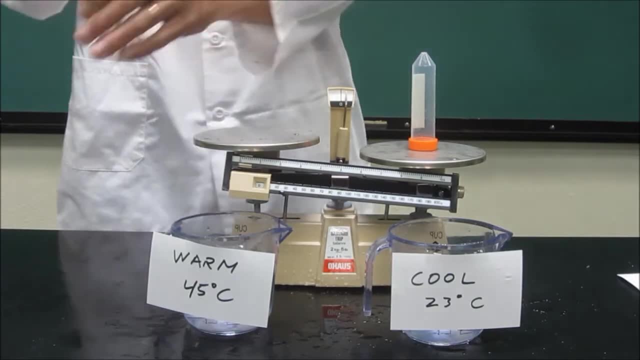 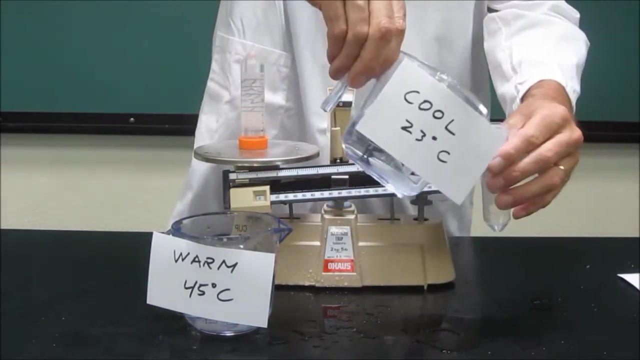 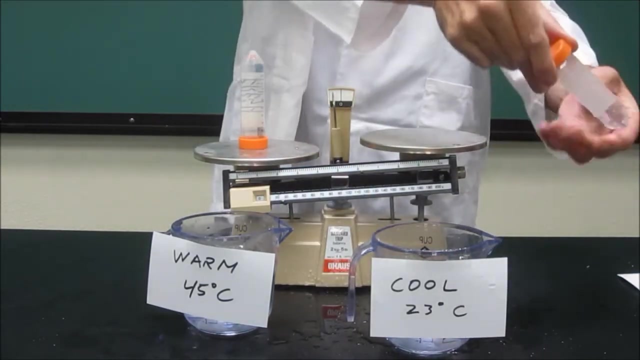 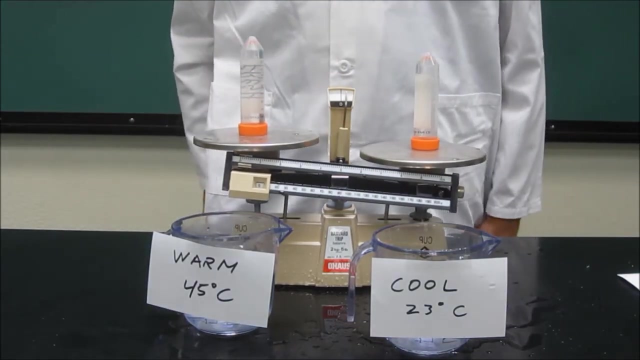 So I'll fill the one with warm water, Put it on the scale, And then I'll fill this one with the cool water sample And put it on the scale, And there you go. The cool water is denser, heavier, for a given amount. 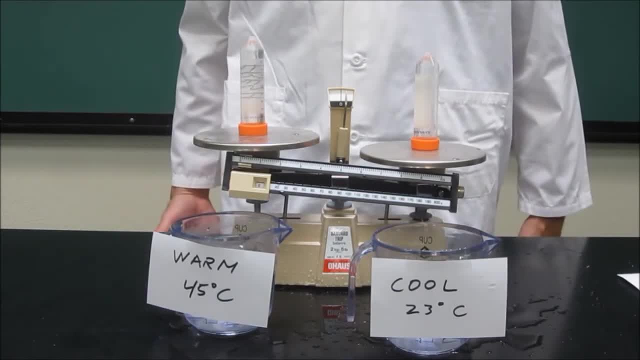 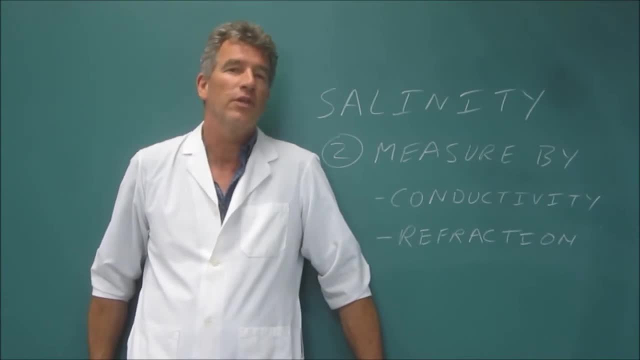 So we've seen that the more salt you add to water, the greater the density. The cooler the water, the greater the density. Okay, we've seen the relationship between temperature and salinity and density. How about how we measure salinity? 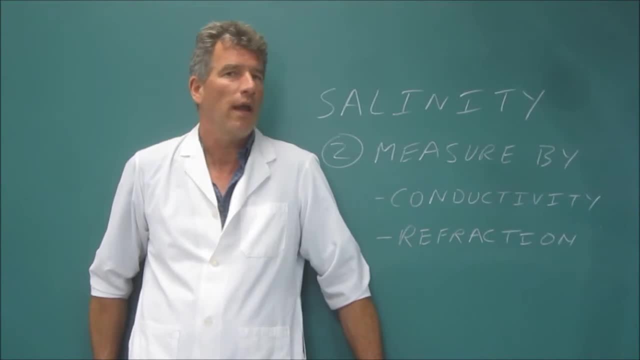 How do we figure out how much salt is in the water? It turns out there's not any one very simple way to do it, But in this lab we're going to use two measurements that are frequently used by oceanographers. First, we're going to measure conductivity, which is how easily water conducts electricity. 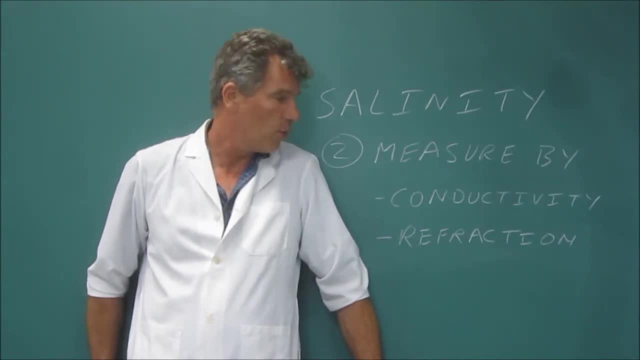 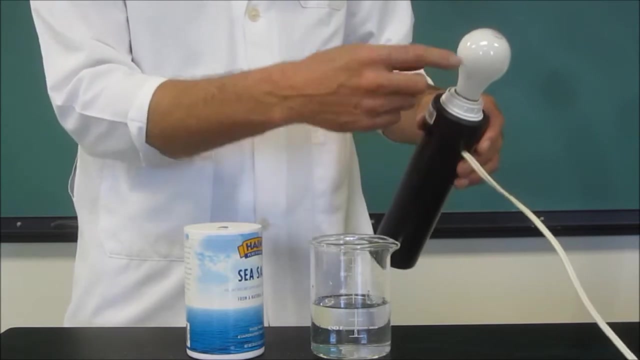 And then we're going to take advantage of the fact that the more salt is in the water, the more it bends light, And the bending of light is something we call refraction. So let's take a look at conductivity first. This apparatus here is connected to a wall outlet with an electrical cord and has a bulb there. 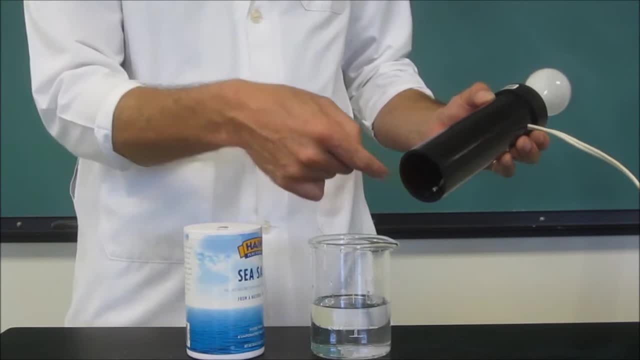 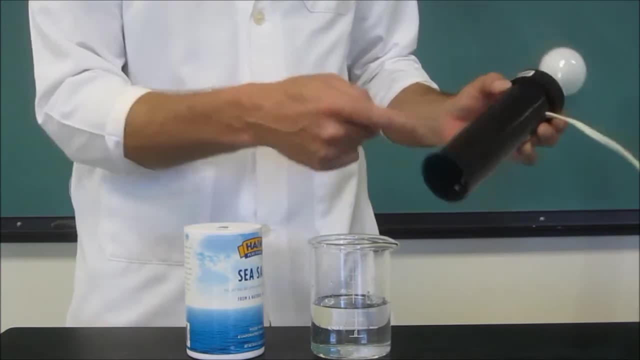 And there are two exposed wires on the inside of the pipe. If I can make an electrical connection between those exposed wires, I can get the bulb to light. It's really important when you're in lab that you not try to make this connection with your fingers or your tongue. 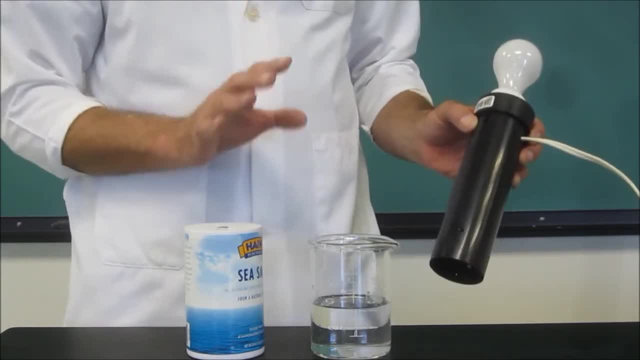 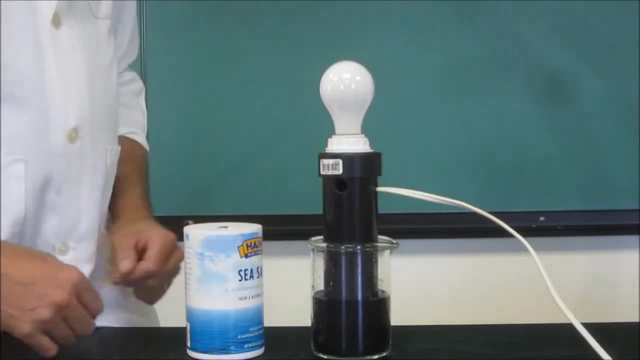 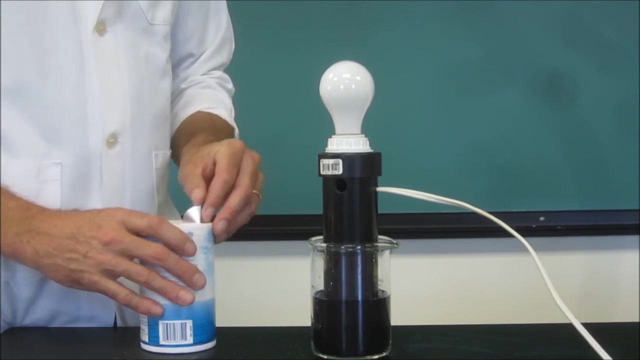 because you could seriously hurt yourself. okay, Let the water do it. Now here's a beaker of fresh water, And when I put the bulb in, nothing happens. okay, Fresh water isn't able to conduct electricity, But salt ions are positively and negatively charged. 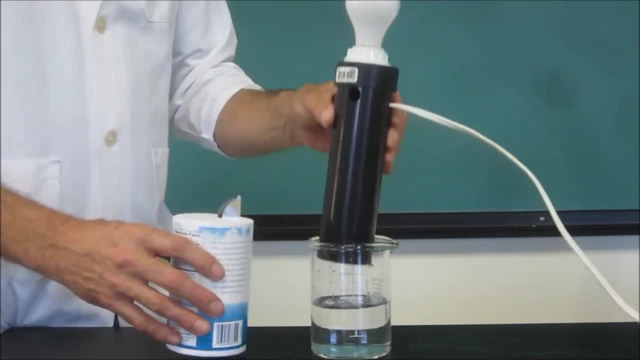 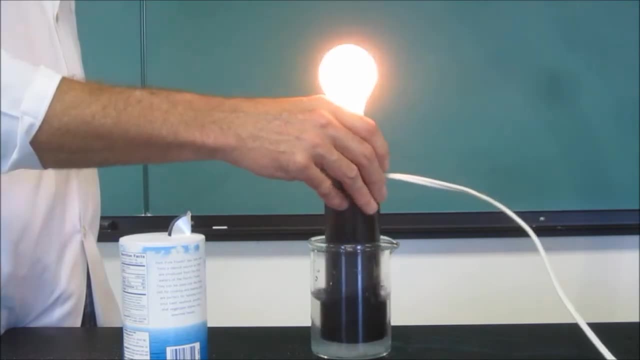 And when they're in the water they can conduct an electrical current. So I'm going to put some salt into my water And then I'm going to stir the salt to get it to dissolve And you can see that it causes the bulb to light up. 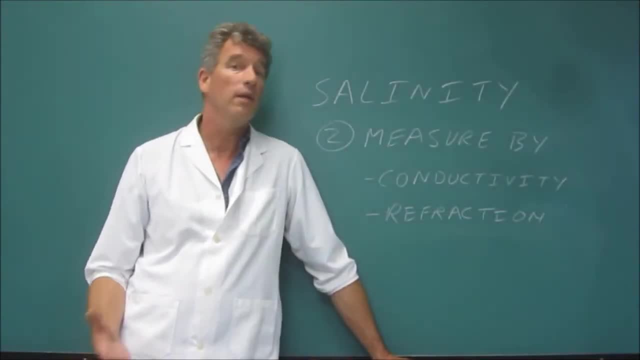 So you just saw that salt water can conduct an electrical current And, as you might expect, the more salt you put into water, the stronger the conductivity. But there's a wrinkle, which is that the conductivity of water also depends on its temperature. 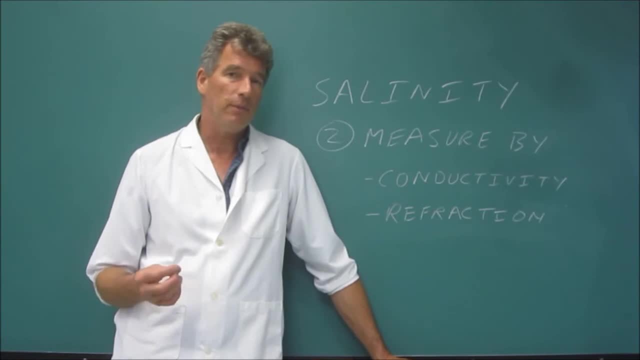 And so in the lab, you're going to explore this relationship, because you need to be able to measure both the conductivity and the temperature of a water sample in order to determine its salinity. So that's the first method we're going to use to measure salinity of water. 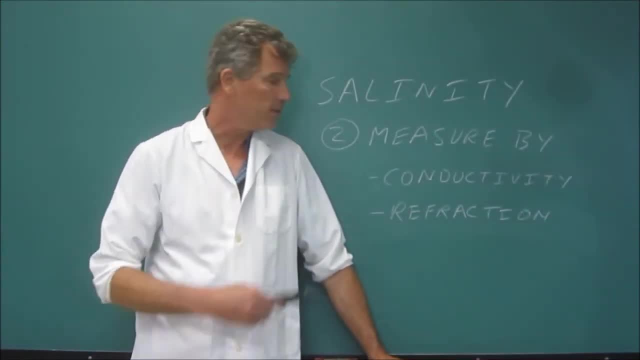 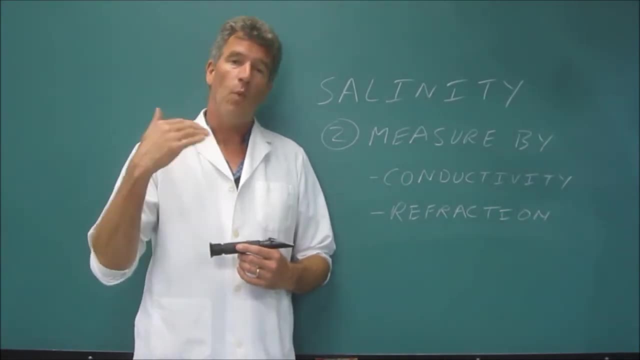 Okay, the next way you're going to measure the salinity of water samples is to use what's called refraction, which is taking advantage of the fact that light, as it passes from one substance to another, will often bend, And that's called refraction. 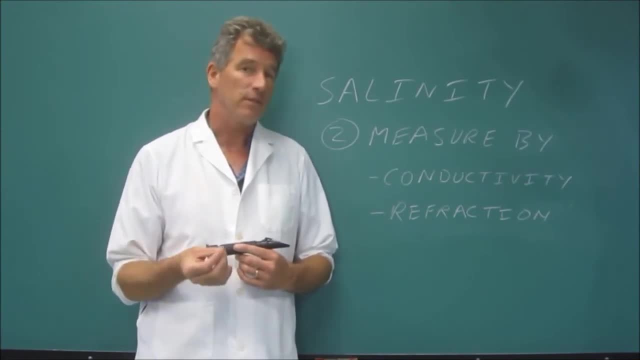 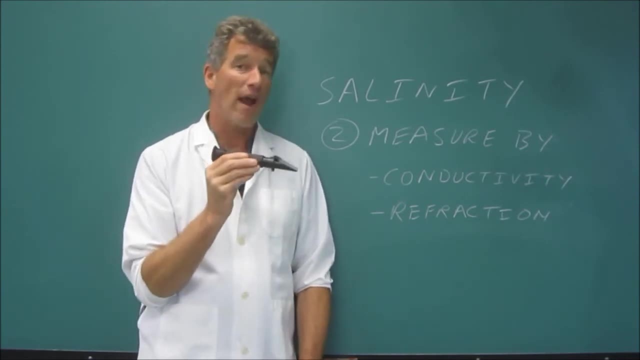 And, as it turns out, the saltier the water, the more it bends when light passes through it. To make this measurement, you're going to use this thing that looks like a black cigar. It's called a refractometer. It's actually going to measure the amount that the light bends. 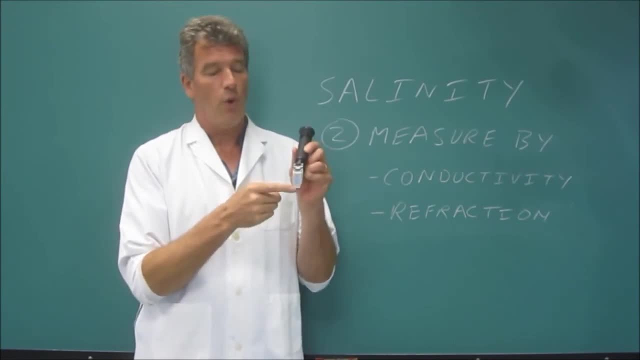 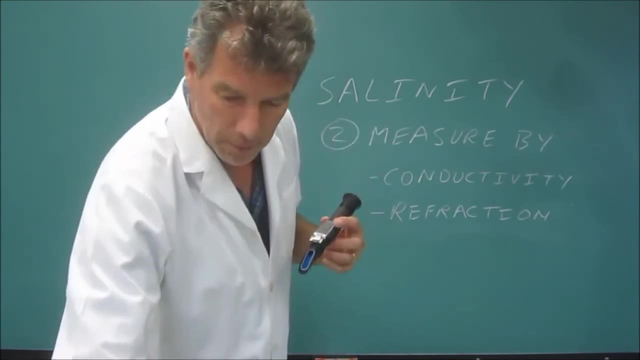 as it passes through your water sample. What you do is you open up the little plastic lid on this And then you're going to take your water sample And there's a dropper that you'll use. Take a few drops of your sample.